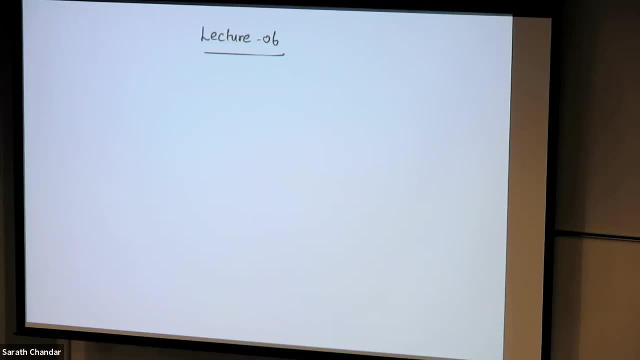 And I want to remind you that. well, I'll send her at an announcement, but I'll still feel it in the class, for extra benefit of people who are attending the lectures in-person and in Zoom. So you'll have three days to ask for regrades. 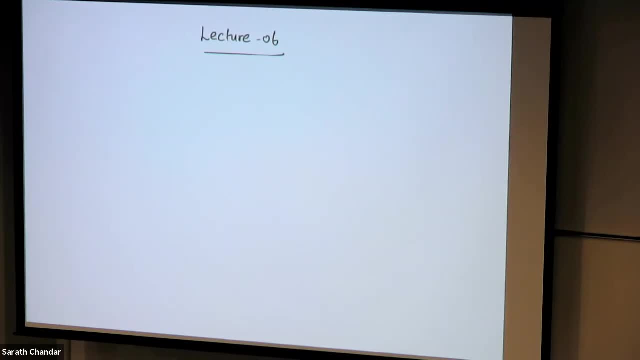 These re-grades must be done only in grade scope. Okay, So you you should not send emails to me or to the TA's asking for re-grades. Please don't do that. You have to just if there's a question which you want answered and I'll just ask in advance. Okay, this is a great picture. Okay, so you should not send emails to me or to a TA's asking for re-grades. please don't do that. You have to just if there's a question which you want answered. 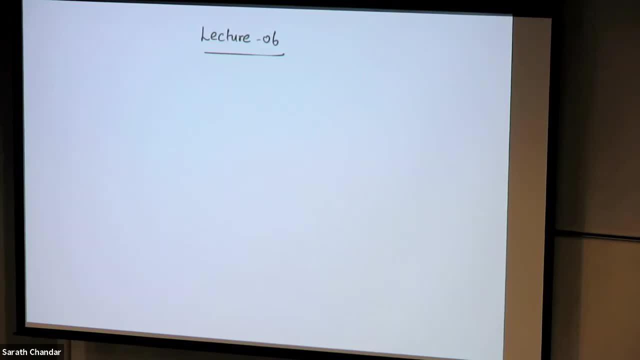 Okay, so you should not send emails to me or to a TA's asking for re-grades. you want to be regraded? you can click regrade for that particular question part and you have to give a detailed explanation for why you are asking for regrade. If there is no explanation, TAs cannot. 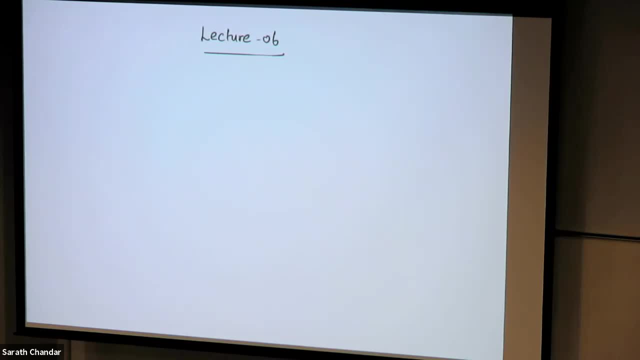 read your mind and try to give you extra marks, okay. So one: please make sure that you give enough explanation when you ask me for your grade. Two, don't ask too many regrades, okay. So I'm saying this because I have seen in the past some students by default go and click regrade for all the 25. 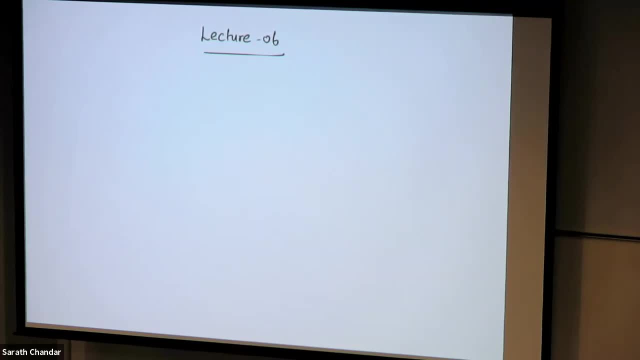 sub questions. Please don't do that, okay? So if we see that you are doing something like the default option of asking for all the questions, regrade- like at least the rules doesn't say that we are going to penalize but it is a bad thing to do. Don't do that like be considerate about TAs time. 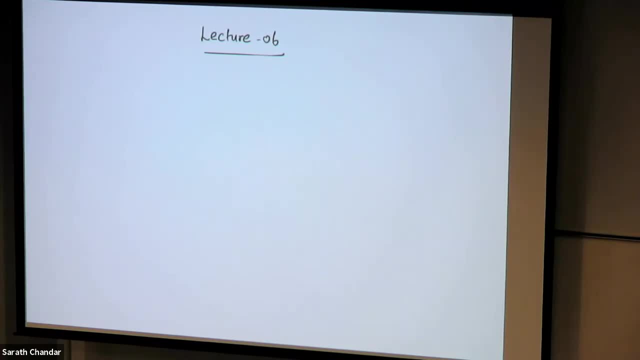 and hopefully these great questions will be answered. So some of the ratings would help you to fix some of the issues that you made in A1. for A2, okay, That is why I wanted to release it much earlier but we couldn't do it like a few days late. but you will see. 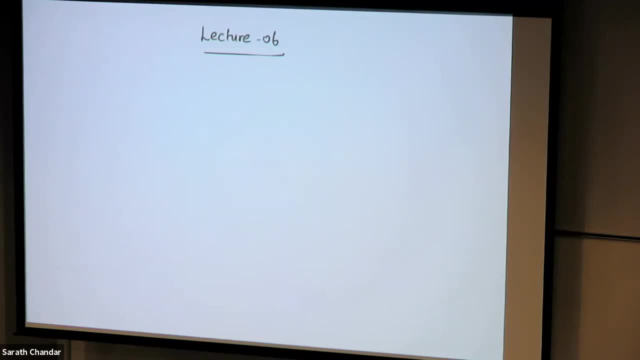 today and you can use that for making changes to your A2. okay, Now, well, while I was talking with you before the lecture, like some of you mentioned that assignment 2 takes a lot of time to train. okay, Well, first of all, I would like to thank you for your time. I really appreciate it. I really appreciate. 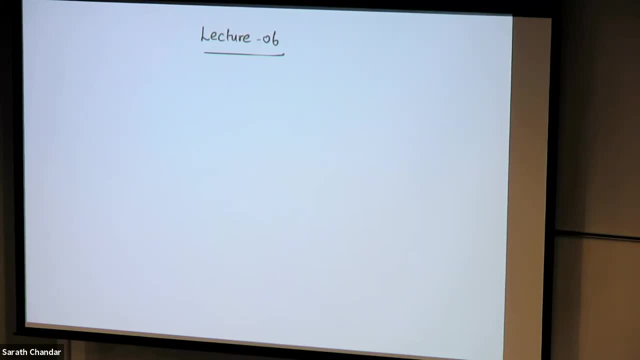 it. First of all, it is normal for machine learning experiments to take a lot of time, but not for assignment 2.. Assignment 2 should not take a lot of time to train, So if it is taking a lot of time then probably you are implementing the things in an inefficient way, okay, So try to avoid for loops. 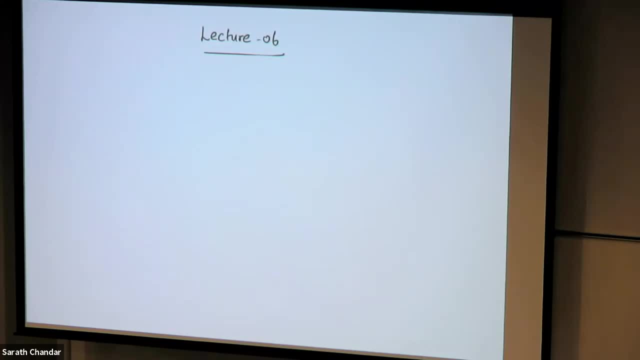 wherever you can like. try to use vectorized operations and matrix operations wherever you can. okay, So now it has some learning curve, of course, but you will learn a lot by doing that, okay, So try to speed up things, For example, like GDM. 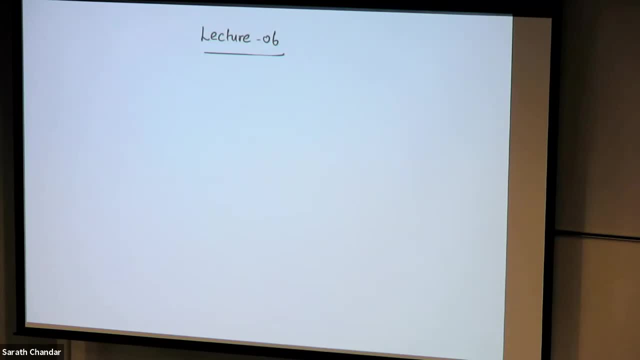 GDM should not take more than few minutes, okay. So if it is taking 40 minutes, 50 minutes for you to train, then probably something is wrong. KNN is going to be extremely slow if you implement it in a very inefficient way. So think about how to implement it in an efficient way. That is also. 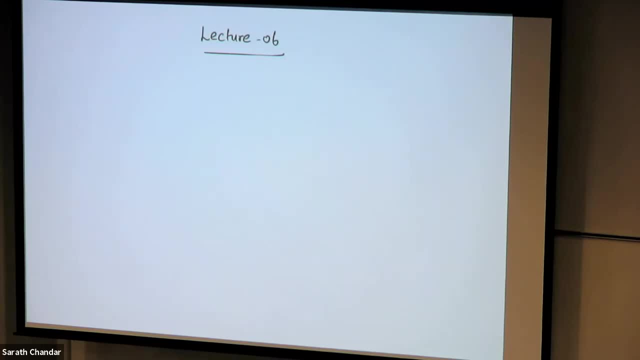 part of that thinking is also part of your assignment, okay, So don't run three hour, four hour jobs for KNN, like it should be. it is going to be slow, but not as slow as some of you are reporting. Okay, now I think we can get started. So just to give you a very quick recap of like what we have seen a couple of weeks back, right, 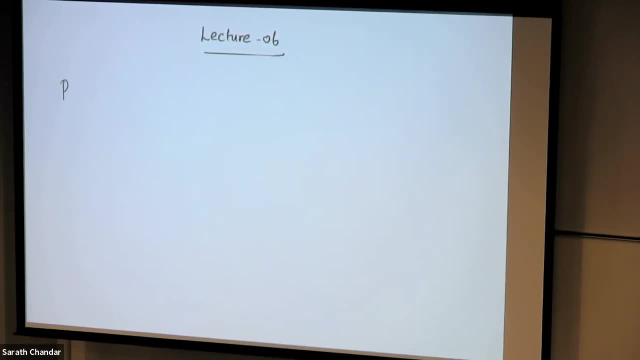 So we looked at probabilistic generative models right Now. to go back even a little further like this is a little bit more complicated, So let's go back a little bit more. So let's go back a little bit more. We started discussing about classification and how there are three ways to do classification like. 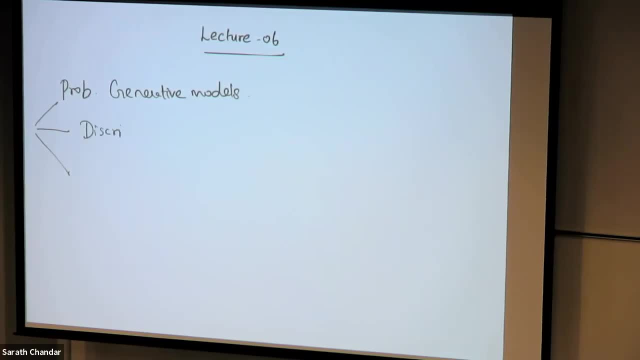 one is generative models, like the. second is discriminative models, right, and third is discriminant based models. So the idea of generative models is to estimate the probability of x comma y. so you could do that in many ways, like: either you can directly attempt to estimate p of x comma y, the 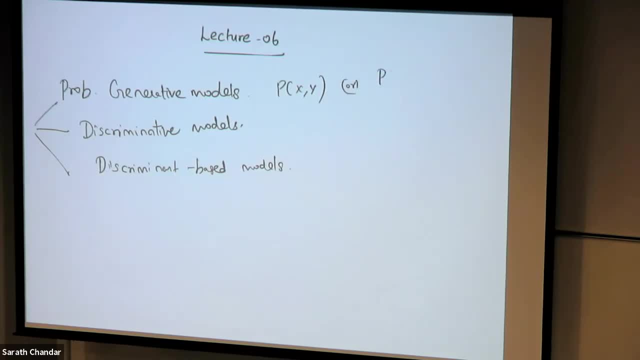 joint distribution or you can estimate p of x given y and p of y and then use the base rule to compute p of y given x, right? So that is what we discussed last week in detail, right like so. specifically, we looked at Gaussian discriminant analysis, GDA and several variants of GDA, and we 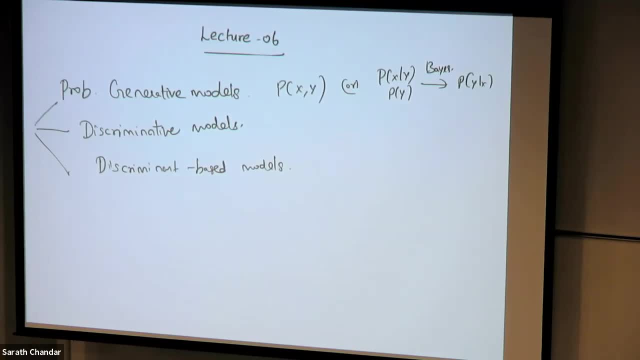 also looked at Naive Bayes, like Gaussian Naive Bayes, like for discrete features, right like so. so that was last week and this week we are going to focus on the second class of approaches, like approach for classification, which is basically the idea of directly estimating p of y given x. There is no joint distribution. 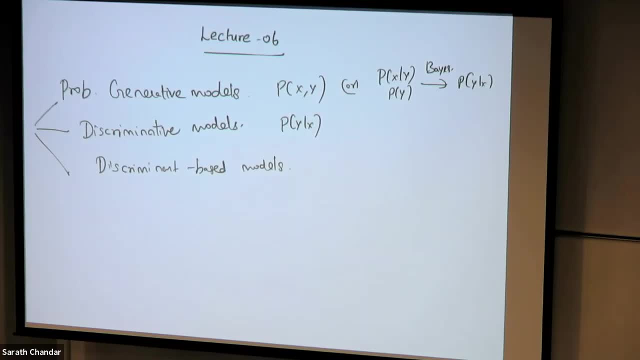 there is no base rule, like it's directly attempted to estimate p of y given x, As you can think, like as you can see here, like it is actually much more simpler than generative model. but there is also this third, simplest approach, which is discriminant based models, like so, where the idea is to estimate. 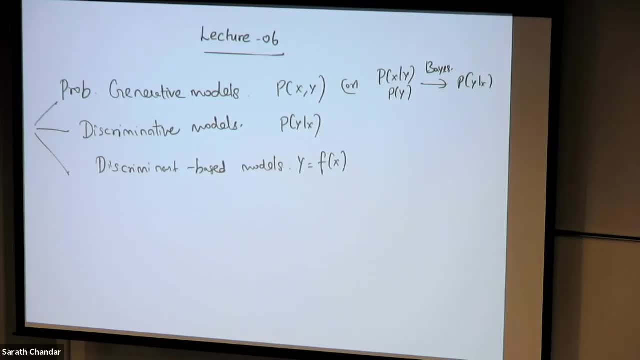 y as a function of x, right, so there is no probability involved. you directly tell me what is the class. Now, we have seen one example for that, right like. so, when we started our discussion on classifier, we saw how to use least squares for classification, right? so so least squares. 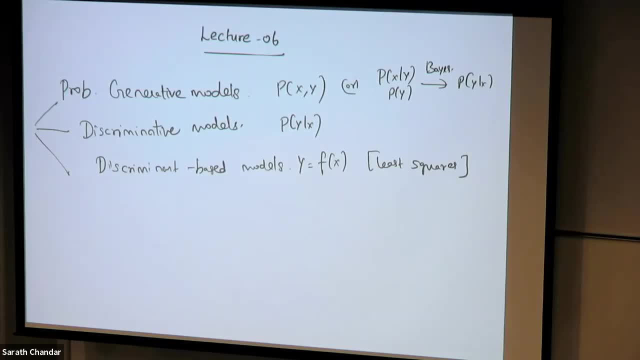 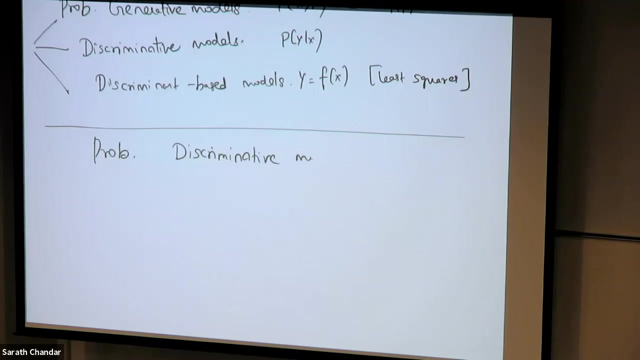 if you think about least squares, it was just taking x and computing some value and thresholding it for class 1 and class 0, right? so it's a discriminant based approach. okay, but we haven't seen any discriminative model, which is the topic for today's discussion. okay, so probabilistic discriminative models, okay. now in the case of 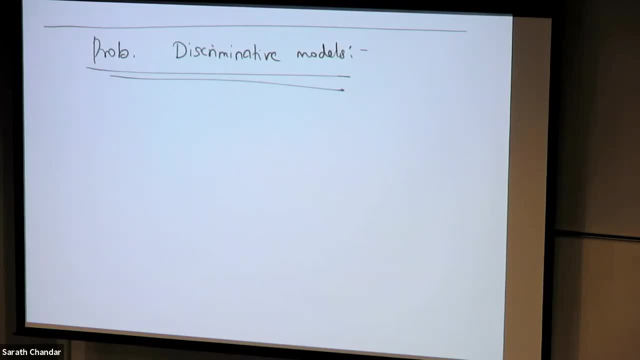 generative models, right. so if you think about, like what we did last week, if you take two class problem, then we had the sigmoid formulation right, like: so: p of c1, given x, is given by sigma of w, transpose x plus w0, right. so where w and w0 in the case of gda, where equations of mean variance. 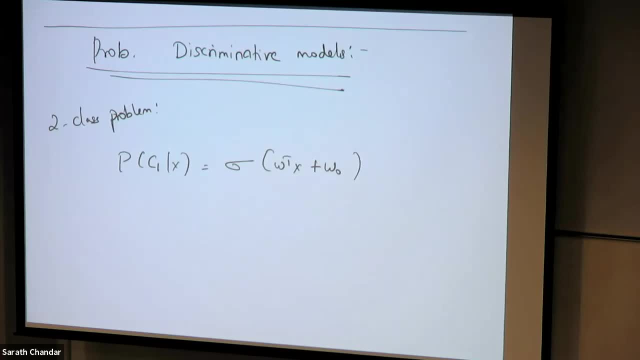 and prior probabilities right. similarly for three. so not three like. so k class problem like where k greater than two, even though we did not derive gda for that. like you had all the tools so that you can do it by yourself like, and we discussed the form of the k class problem right. 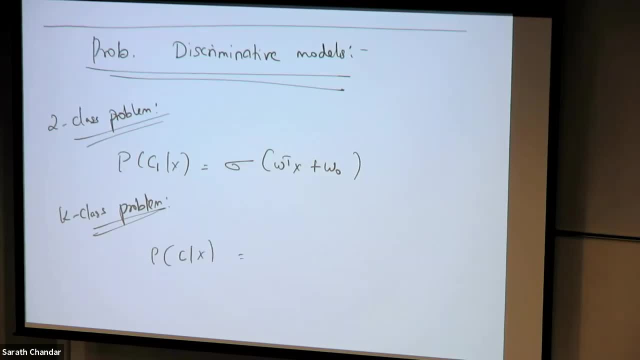 like so in the case of k class, problems like the probability of c given x was given by softmax function of w. transpose x plus w0 right where softmax is basically like generalization of sigmoid, but for many classes right now, in the case of generative models, 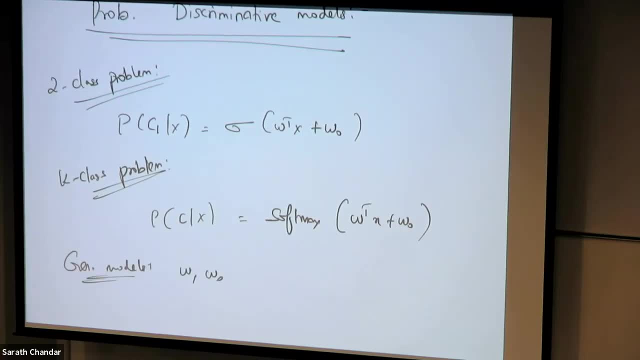 so both w and w0, the functions of mean covariance and prior probabilities, are the same. right now, the idea of discriminative models is really simple. like, instead of treating these w and w0 as functions of mean covariance and prior probabilities, how about we just throw all of them and treat w0 and w as some parameters, if you want to estimate? okay, so that is what the 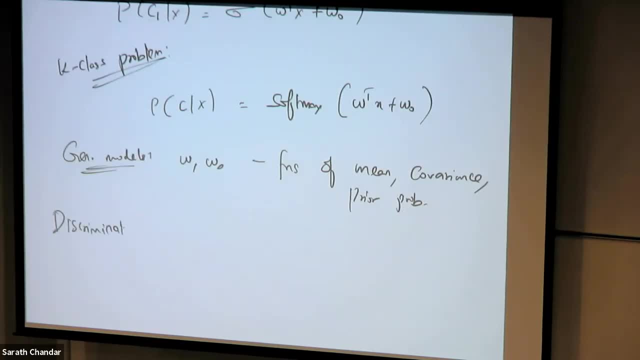 discriminative approaches are okay. so now we are going to forget about the gaussian assumption that we had and the mean and covariance estimation for the gaussian and other stuff. we are going to assume that w and w0 as a vector of parameters- okay, and we are going to directly learn w and w0 from the data by using maximum likelihood. 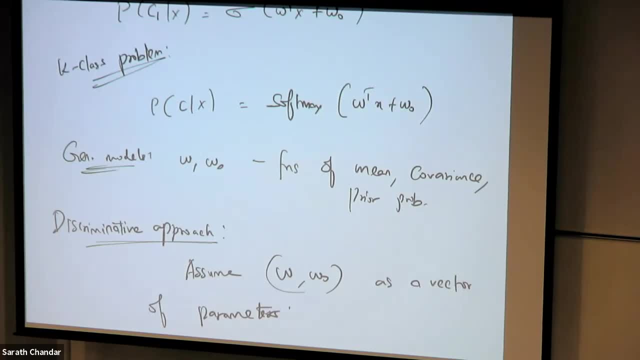 is that clear? now, why is this interesting when compared to gda? so there are many reasons like so. for example, how many parameters do we need? if i treat, let's take p of c1, given x is equal to sigma of w, transpose x plus w0. okay, and there are m features. 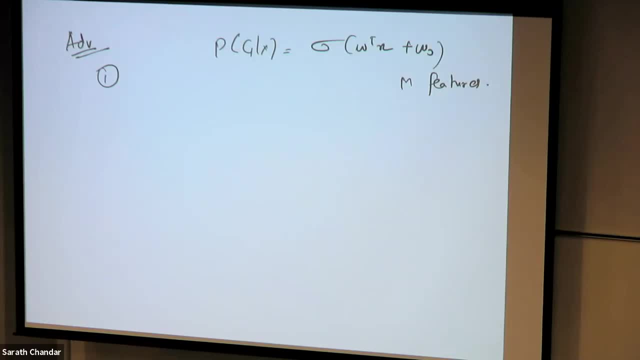 now, how many parameters do i need for this discriminative model? m plus one, just the parameters that you have here, right like. so, first of all, it only requires m plus one parameters. okay, well, compared to something like gda, which requires m parameters for mean m into m plus one by two parameters for covariance. 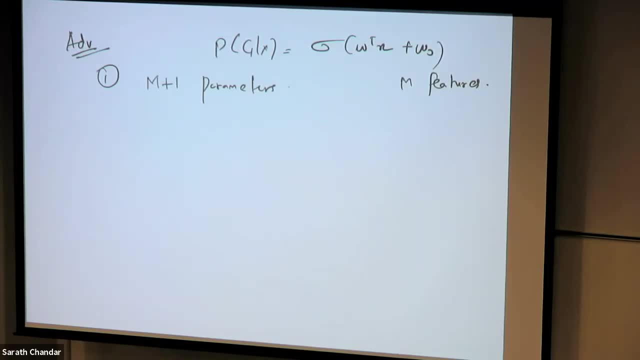 and another m minus one, m minus one or approximately order m parameters for the prior probabilities, right, so it's a lot of parameters with generative approach. however, with this discriminative approach, the number of parameters is much lesser than the number of parameters in generative approach. 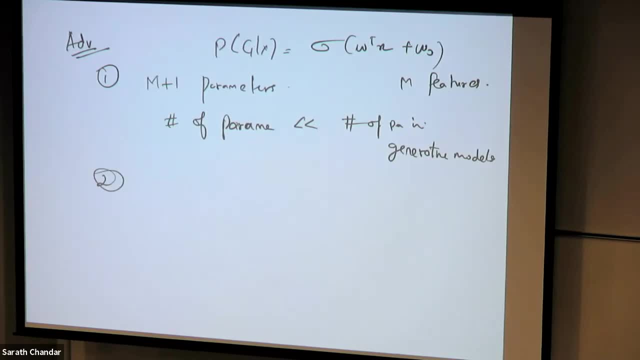 okay. also, the second big advantage is we don't have any restrictive assumption about the class distribution here. right like so in the case of gda, we made the gaussian assumption. now, when you have discrete data, you have to make a bernoulli assumption. now, what if the data doesn't? 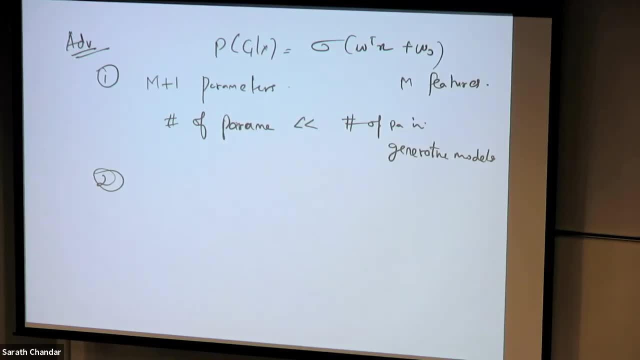 follow generative, like like a gaussian distribution or or a bernoulli distribution. right like so. when there is a distribution mismatch which we could never figure out first of all. right like so, then you're going to get bad performance. now you don't know if this bad performance is because of the model. 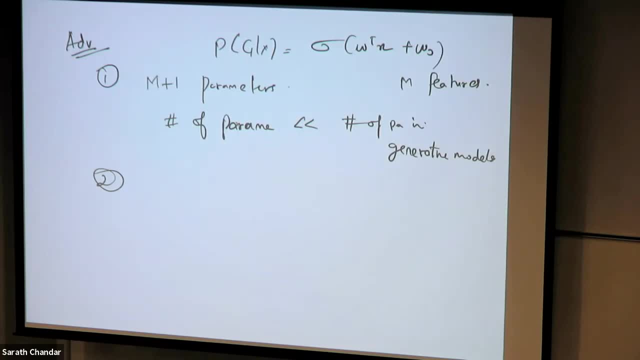 or because of this assumption right. on the other hand, discriminative models might have improved performance. okay, when the class conditional density assumptions that we had right, like the assumption that the class conditional density is gaussian, is a poor approximation to true distribution. is that clear? so in those situations it is just safer to do discriminative approach because it. 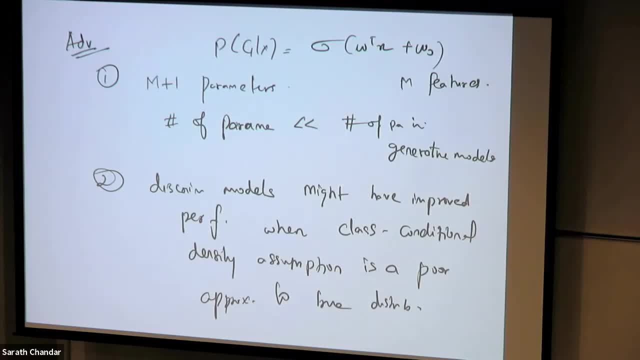 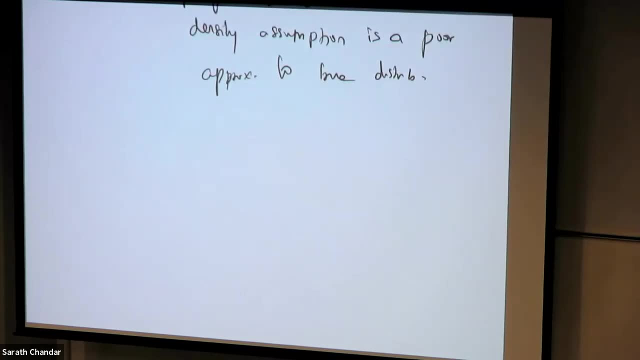 doesn't make any assumption about the distribution, like, so it will not have such mismatches. is that clear? so now we are going to see our first discriminative model, okay, which is really really simple, like: okay, so we are going to call this as logistic regression. okay, so logistic regression is defined by one equation, so p of c1 given x. 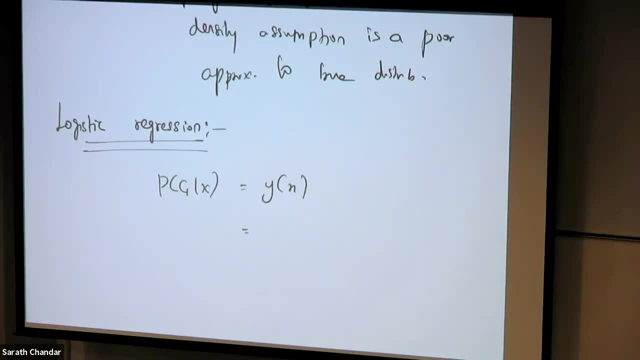 is equal to y of x. okay, which is basically sigma of w, transpose x. is that clear? so i have included the w0 inside w, like, so that the equation looks simpler. okay, so there is a bias, but we are not showing it here now. why is it called logistic regression, like? 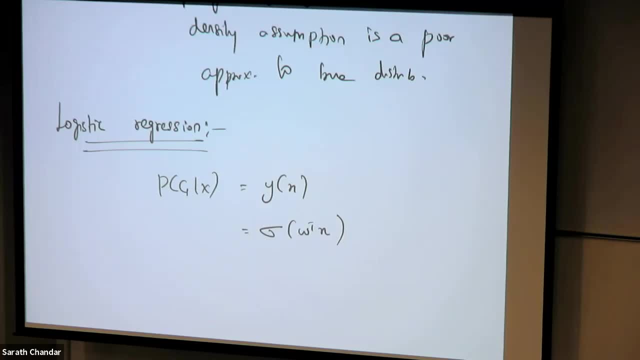 while it is a classification algorithm, right, like it's, the name is just a misnomer. like it's a classification algorithm, okay, but it is called regression, logistic regression, because it looks like regression followed by a logistic sigmoid function. okay, so so don't get confused that this. 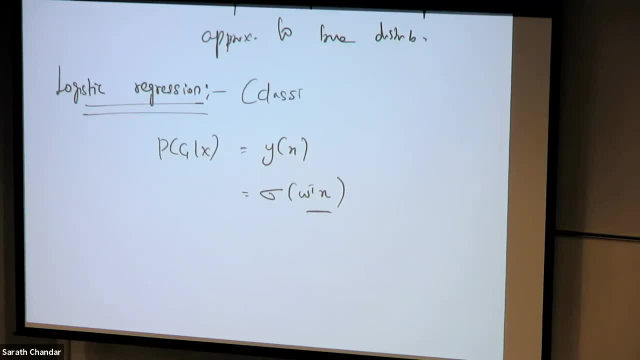 is a regression algorithm. this is a classification. poor naming, okay. so now what would be probability of c2 given x in binary? we are in binary class setting right. so, like what would be p of c2 given x, it's just 1 minus p of c1. 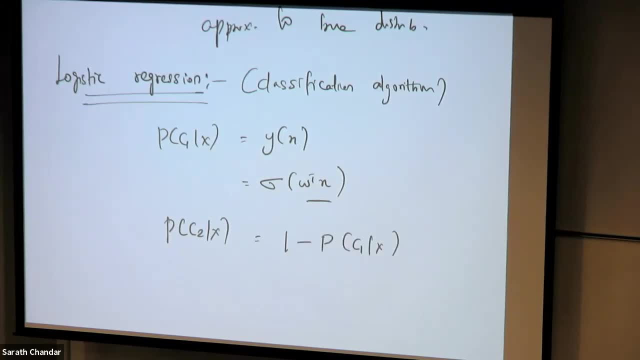 right, so the sigma here. we have already seen the sigma, so this is the logistic sigmoid function. okay, now is it clear? like it's it's a really simple model, like it's a sigma of w transpose x, but the parameters are w. now our only job is to estimate these parameters, w, from the data. 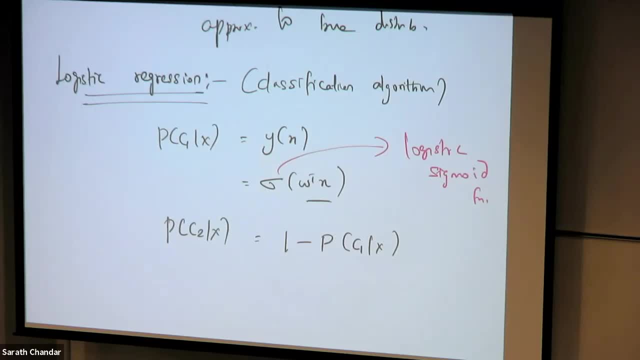 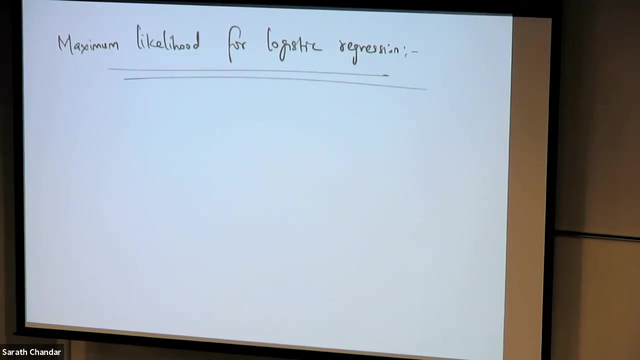 okay now to do that, like we're going to repeat the process again. like we're going to repeat the process we did last week, but it is going to be much more simpler today. okay, so we are going to do maximum likelihood estimation for logistic progression. so, as a quick recap for maximum likelihood, right like so, if you remember our discussion on gda, 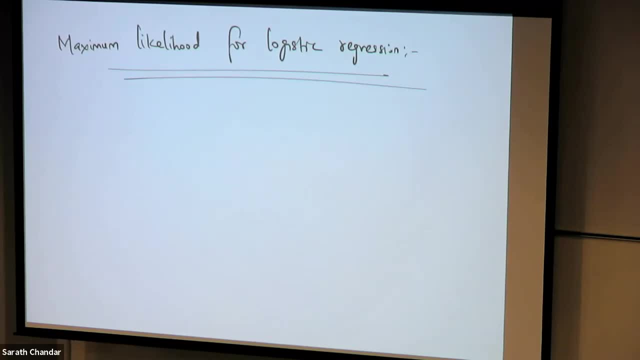 so, whenever you have a probabilistic model and you want to estimate the parameters of this probabilistic model, you want to estimate the parameters of this probabilistic model. like so, one objective function that you could use is the maximum likelihood. right, like so, you want to maximize the likelihood of seeing this data from the distribution. so any model which gives 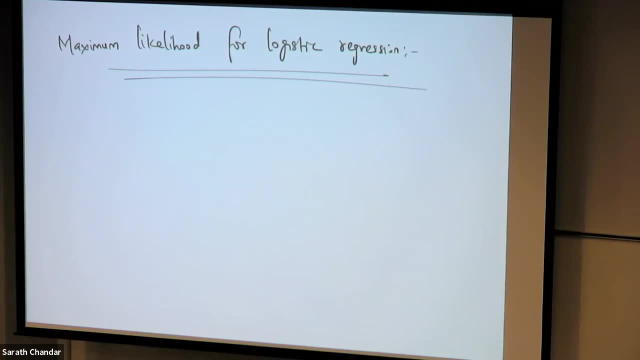 maximum likelihood is probably a good approximation for the underlying probability distribution. right, so now, to do that, we need a data set. so let us assume that we have some data set which is a bunch of xn and tn. okay, where you have capital, n, number of examples. okay now, where tn is going to be either zero or one. 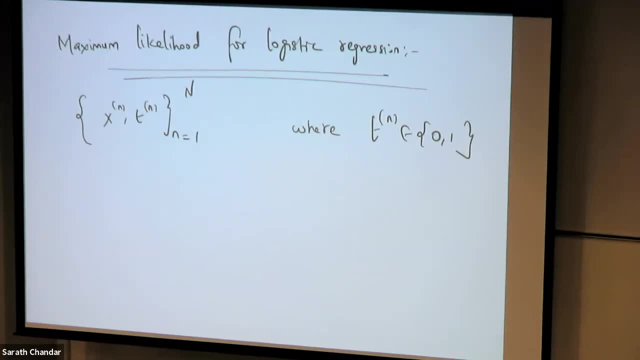 okay, now we just care about probability of t given w right, so we want the probability of the class given some parameters. okay now, this is given by for the entire data set. like you, you will have product right. so this is given by for the entire data set. like you, you will have product right. so 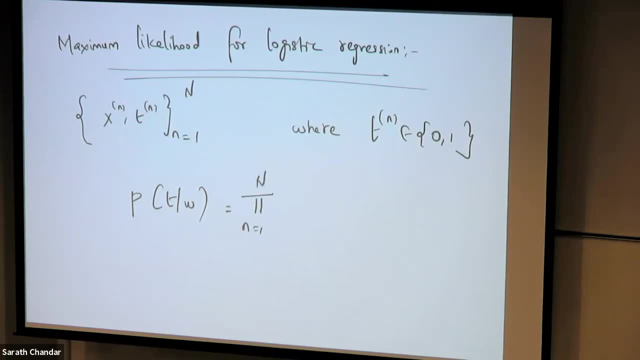 because of the iid assumption. so it's going to: product over n is equal to 1. to capital n: okay, so my probability is going to be yn if t of n is equal to 1. right. if t of n is equal to zero, my probability is going to be 1 minus y. so 1 minus y of n for 1 minus t. okay, so now we have seen this. 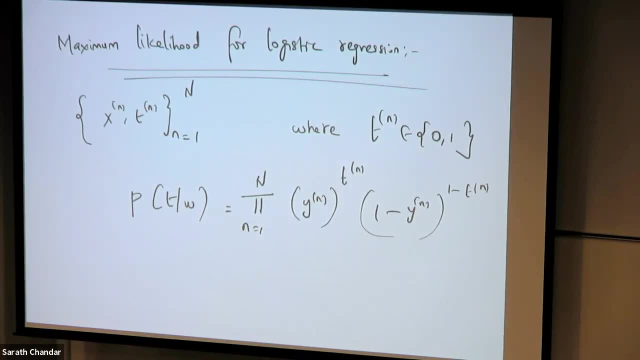 equation even last week in different form, right like so. now we are interested in knowing the probability of the class. so if class is 1, then this term is zero. sorry, this term is anything so 1, so this term disappears. you only have this term, so you get yn. so yn is basically sigma of w. 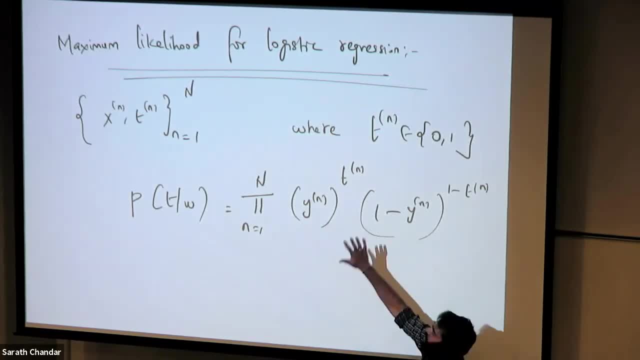 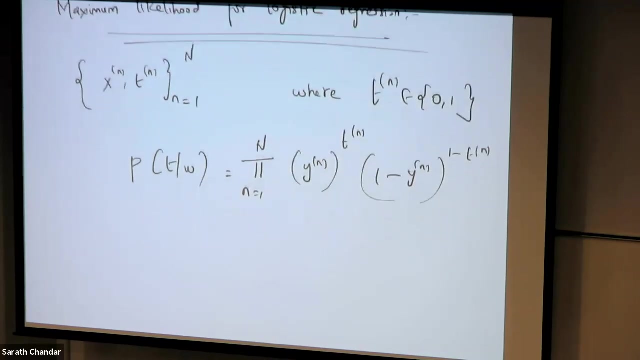 transpose x, right, if class is zero, then this one disappears. you only have this. so 1 minus 0 is 1, so is 1 minus y. so this is just a compact notation for both the probabilities, like so if it is class 1 or class 0. okay now where t is basically all the examples classes and y of n is basically p of c1. 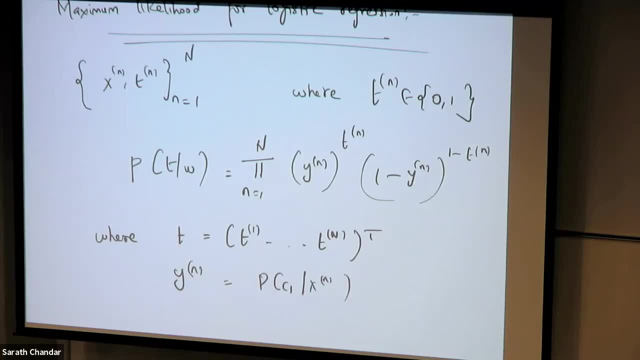 given x of n. is that clear? now i have the probability, given a data set, i just need to estimate this probability, which is the likelihood, and maximize this right. so now, instead of maximizing the likelihood, we often maximize the log likelihood so that this particular product becomes a sum right. and again, if you remember our discussion, 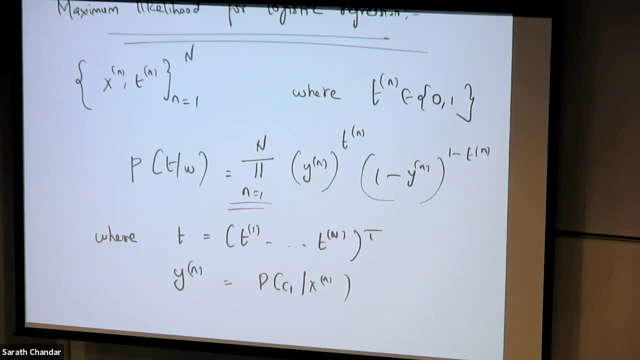 last week. instead of maximizing the log likelihood, i can minimize the negative log likelihood. okay, because when we do gradient descent, we always care about going to the minimum, not maximum, right? so there's, it's just a convention. okay, so you can do whatever you want, but what we are going to do, 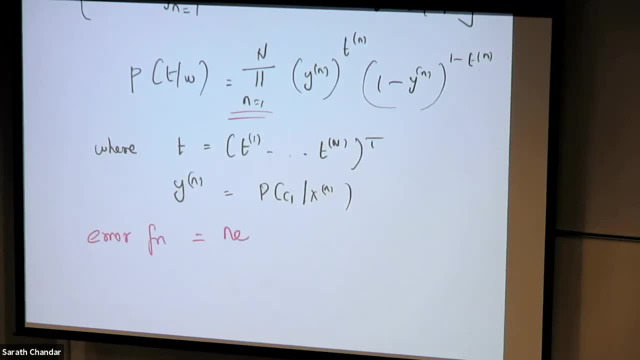 today is our error function is going to be negative log likelihood. okay, uh, maybe a quick quiz. so what are the other error functions that we have, okay, seen so far in this course? least square, yeah, anything else, yeah, mse and least square are- they are same. yeah, r must see. okay, they are all same. 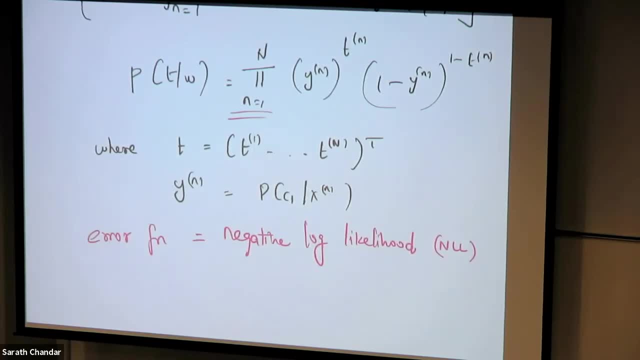 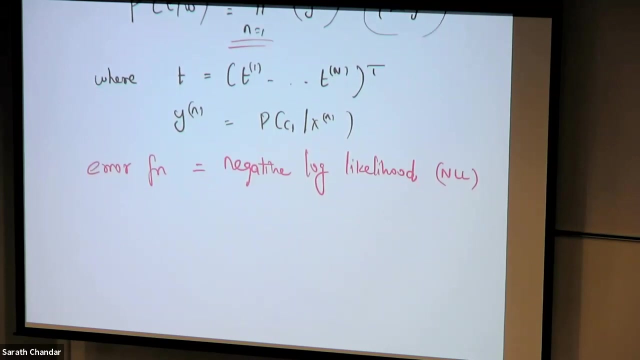 anything else. well, we have not seen anything else like so. this is a second error function. like so, we will see many more error functions in the future, but, like so far, we have seen mse and negative log likelihood. okay, so now the error function e of w is given by minus lon p of t, given w. 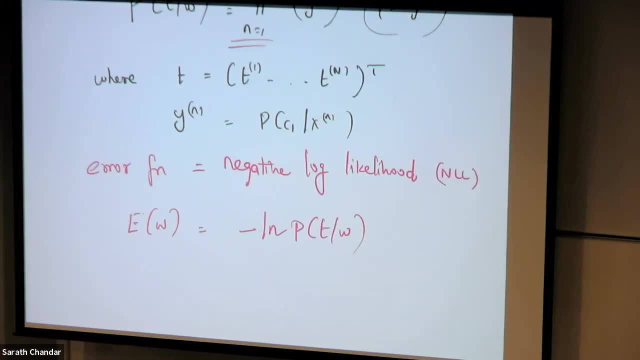 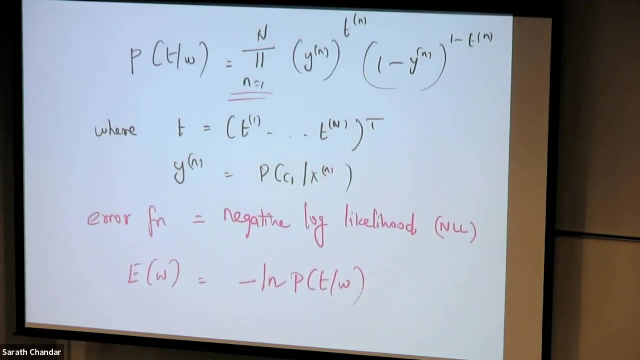 right. so i want to maximize the probability of t given w for the data set, which is equivalent to maximizing lon p of t given w. instead, i'm going to minimize minus lon p of t. okay, now, the advantage of this notation is like i'm just going to do minus instead of the product. 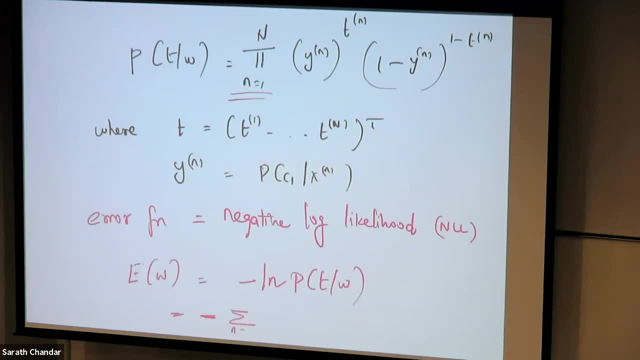 i have summation, so summation over n is equal to one to capital n. okay, you have p of n lon y of n plus one minus t of n, lon one minus y of n, right? so i just took this equation, which is lon a- b. it became lon a plus lon b. 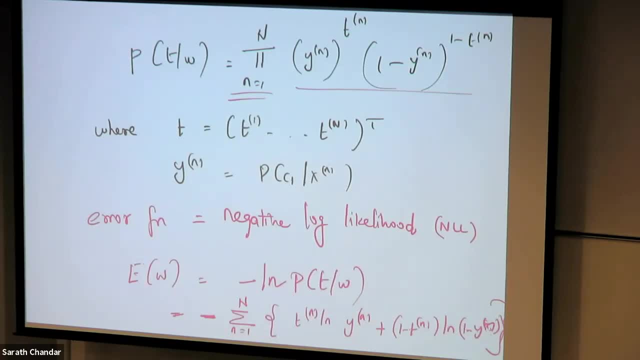 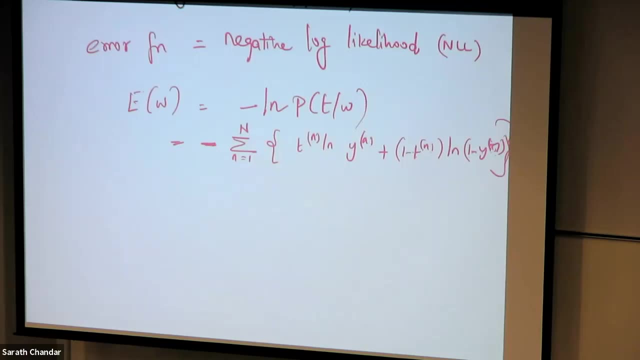 and when you do lon a, power x, it's x, lon a. okay. so basic logarithmic operations. so this is my error. function now: okay, where y of n is given by sigma of some a of n, okay. but again a of n is given by w, transpose x. 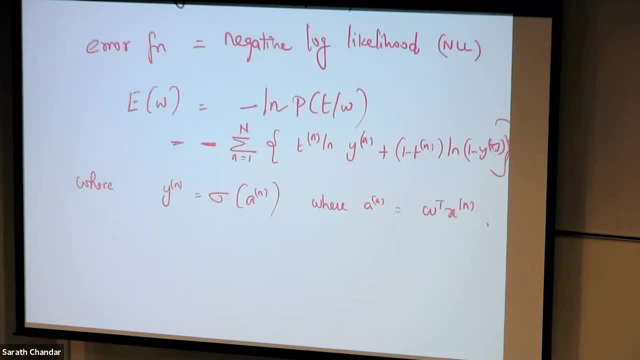 of n. is that clear? any questions so far? so all i have done is like i have constructed this negative log of n and i have constructed this negative log of n and i have constructed this negative log. likelihood error function. okay, now we know the routine like so. 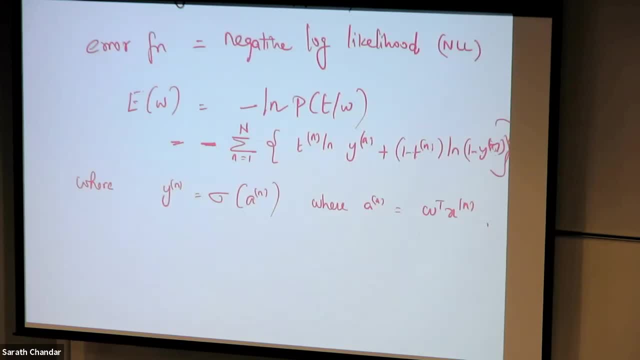 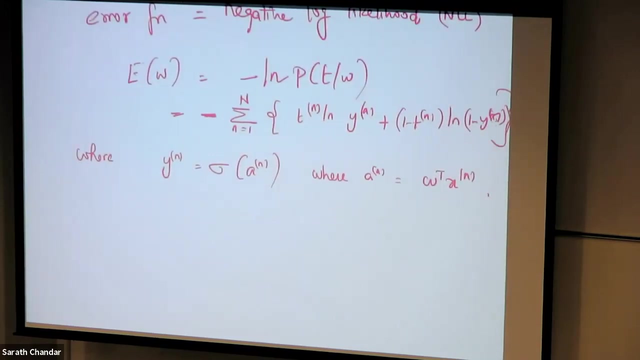 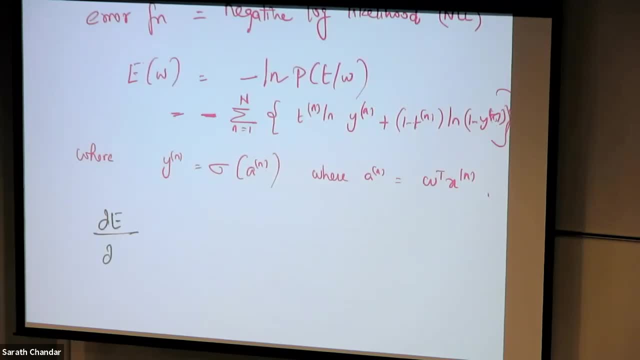 E by dou. sorry, we are interested in dou E by dou W right Now. dou E by dou W. we are going to come take this and we are going to compute dou E by dou W. but do you see W in the equation? No, right, but there is W inside, right, like so this equation is a function. 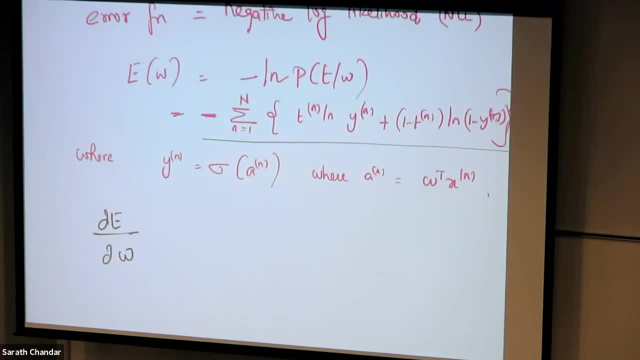 of Y. Now, Y is a function of A and A is a function of W, right, So we are going to use chain rule for computing this derivative. So this is basically summation over: N is equal to 1 to capital N. okay, dou E by dou YN, So it is partial derivative. So dou YN divided by: 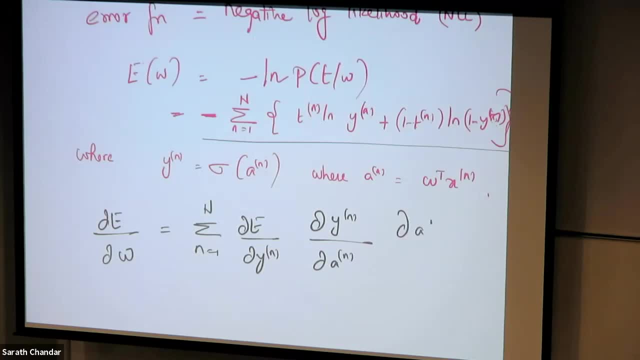 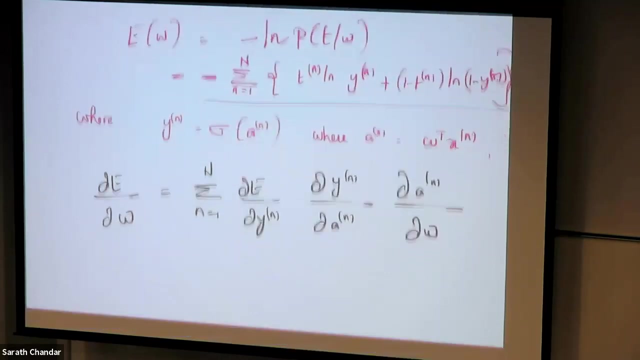 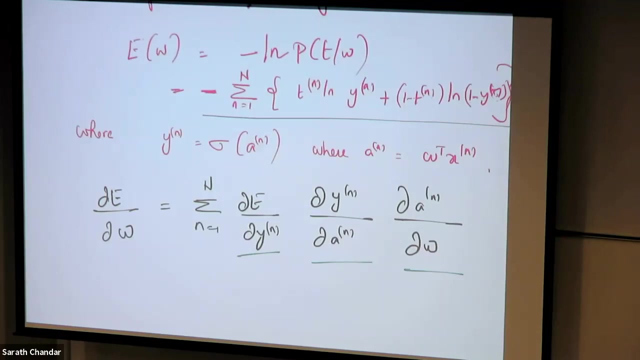 dou A of N, dou A of N divided by dou W. right, So it is just basic chain rule, like so to compute dou E with respect to dou W. Now we just need to compute these three terms separately and put them together. we have our gradient, okay. So first let us do dou E by dou Y of. 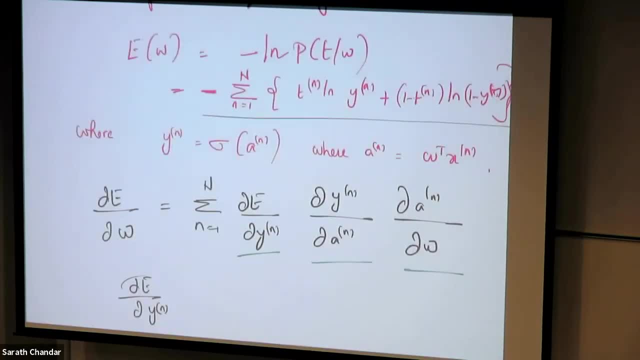 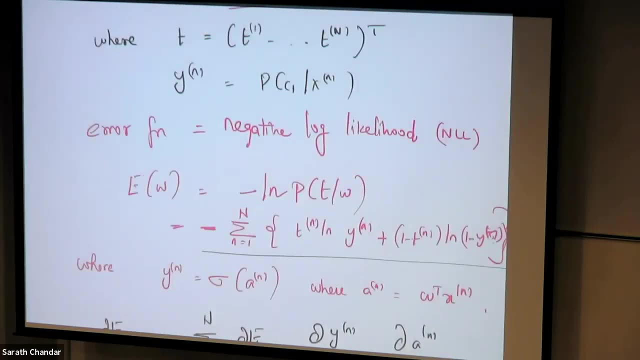 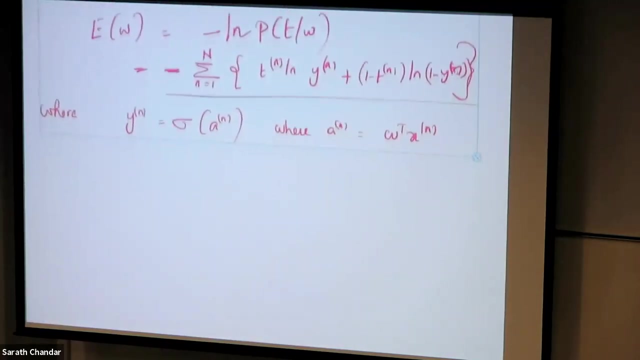 N. Given that I do not have enough space, I will just move to the next page, okay? So let us actually take what we need. Okay, this is what we have Now. what is dou E by dou Y of N? So now let us just do it for. 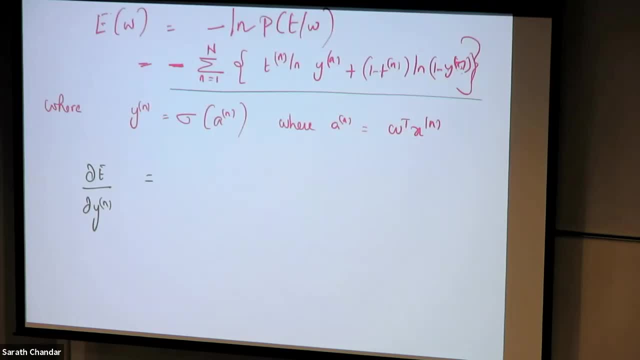 one example, okay, So when you have only one example? so then this is going to be minus T of N. You differentiate ln- Y, so what do you get? 1.. 1 by Y, right? So by Y of N N. 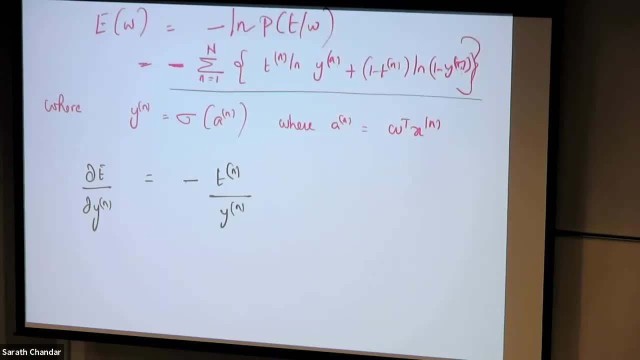 1, by Y 1,, so by Y of N. 1 by Y okay 1,, so by Y of N 1, 1, 1 by Y 1,, so by Y of N. 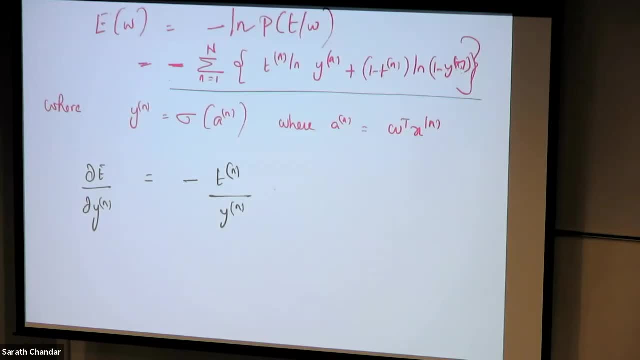 1, so by Y of N There is a minus. okay, 1 minus T of N divided by ln 1 minus. so when you differentiate ln 1 minus Y, you get 1 minus Y. Now you differentiate this again, you get a minus 1, so this becomes: 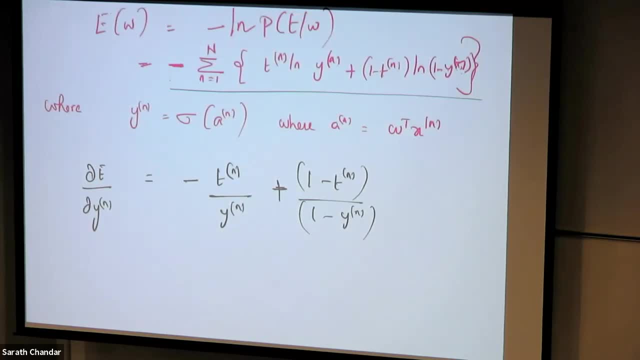 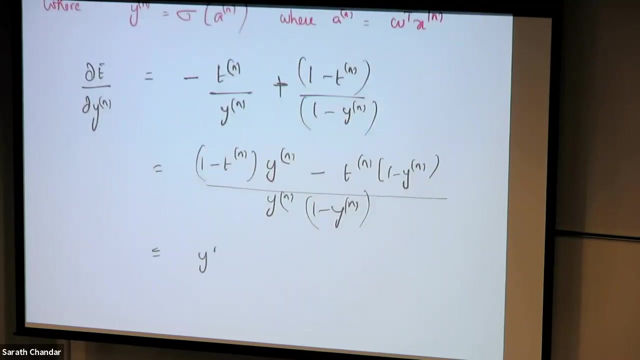 plus. Is that clear? So now just do the basic, like restructuring. so this becomes 1 minus T of N times Y of N. so this is the second term, minus T of N times 1 minus Y of N, divided by Y of N, into 1 minus Y of N. Okay, now this is basically Y of N minus T of N, Y of. 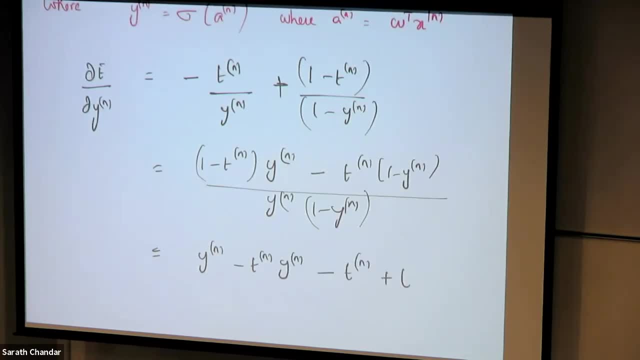 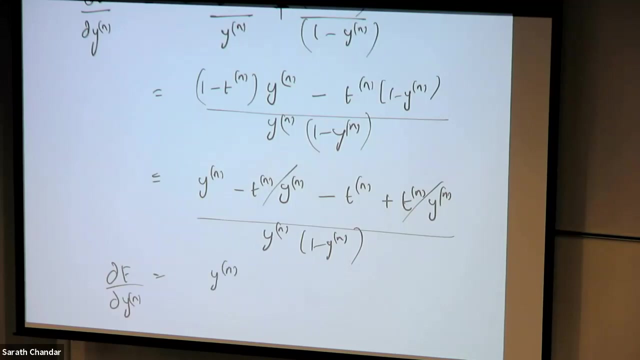 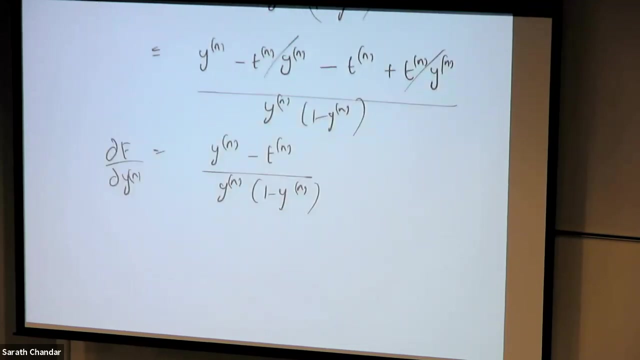 N minus T of N plus T of N, Y of N. This cancels, so you get dou E by dou. Y of N is equal to Y of N minus T of N, divided by Y of N multiplied by 1 minus Y of N. Is that clear? Okay, now the next part of the 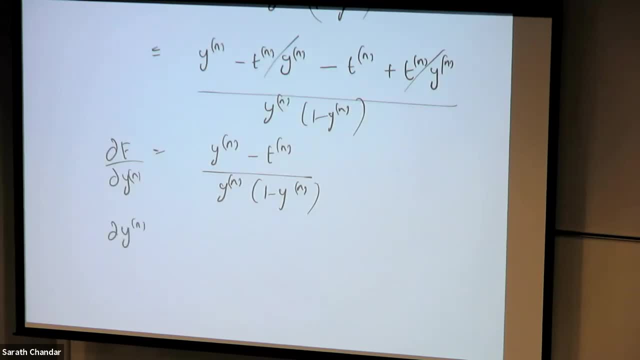 chain rule. so we want dou Y of N divided by Y of N, minus T of N, Y of N. So this is Y of N divided by dou A of N. So if you remember, let's put it here. so Y of N is 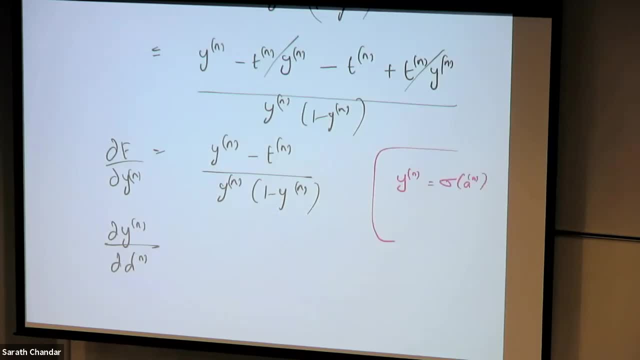 given by sigma of A of N. where A of N is given by W, transpose X. right Now, what is the differentiation of sigma? We have seen that last week when I introduced the sigmoid function, It's just sigma into 1 minus sigma. okay, So that's, it's easy. So it's sigma into 1. 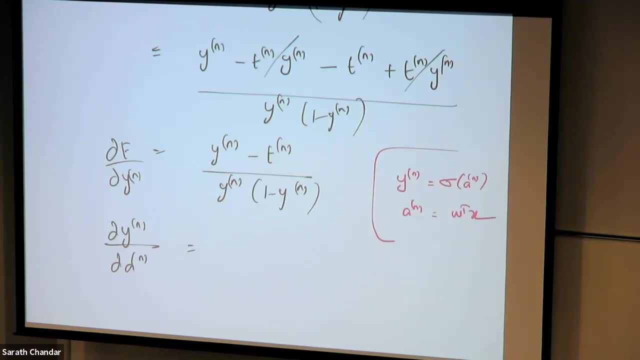 minus sigma. So in this case it's basically Y of N into 1 minus Y of N. right? Now the final part. dou A of N divided by dou W, What is it? What is it? What is dou A by dou W? It's just X, right? So it's X of N. Okay, now we can put together. 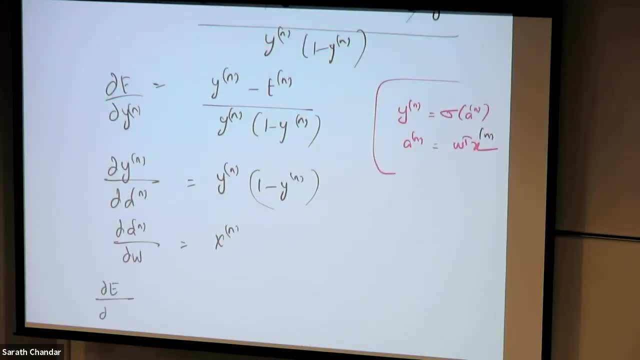 all these things. okay, So my dou E by dou W is going to be: summation over N is equal to 1 to capital N. okay, The first term dou E by dou Y of N, So Y of N minus T of N divided. 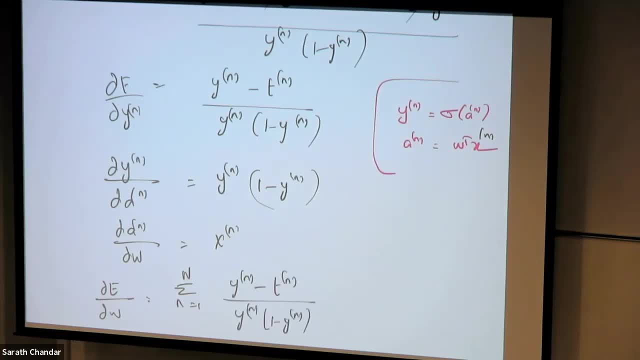 by Y of N into 1 minus Y of N multiplied by the second term, So Y of N into 1 minus Y of N multiplied by the third term, which is X of N. okay, So now you see that these things get cancelled. okay, We have actually a very simple update. 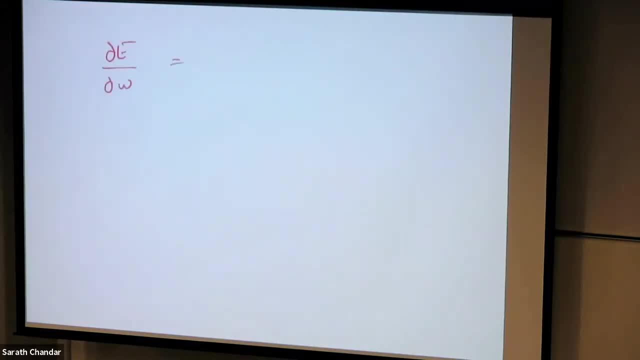 rule. So dou E by dou W is equal to summation over N, is equal to 1 to capital N, Y of N minus T of N multiplied by X of N. Okay, Is that clear Now? have we seen this equation before? 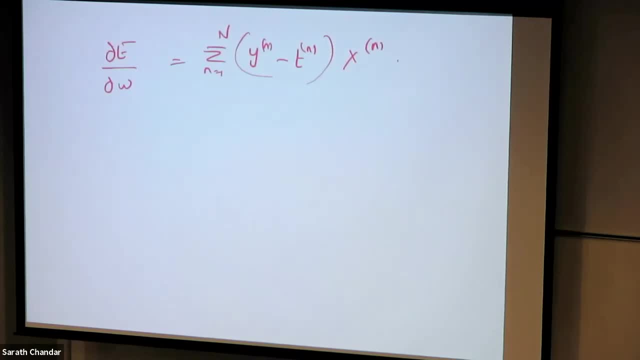 Where? No, We had a closed-form solution for GDA. Oh, first of all, we don't have a closed-form solution here. Where have we seen this gradient update? yeah, Who is anybody from the Zoom call? Okay, some people are going back in their notes. 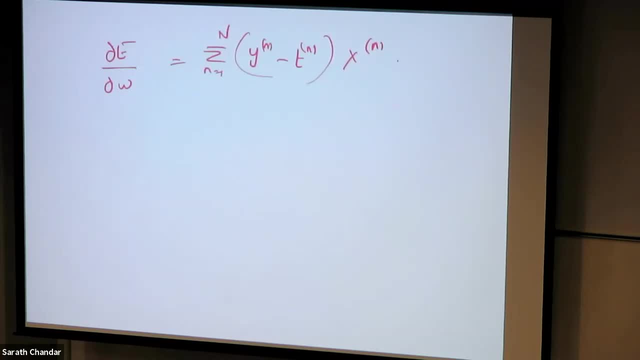 Can you speak a bit louder? I'm not really sure. Okay, Sorry. No, we have seen same gradient equation before. Is it gradient descent or naive bias? No, No, we did not do gradient descent for naive bias. So can you recall, like the gradient for linear regression? 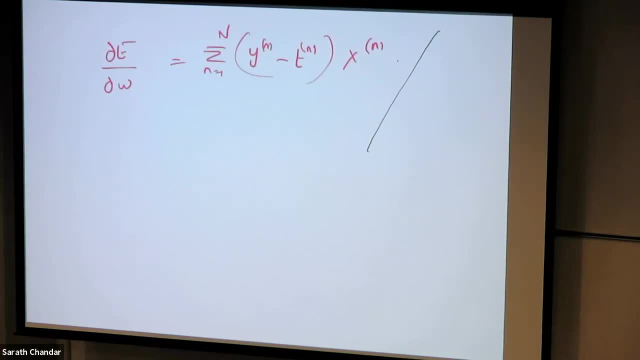 So in the case of linear regression you had an error function which was basically Y of N minus T of N, the whole square 1 over 2, right Where Y of N was just W, transpose X of N. So when you wanted to do linear regression, gradient descent for linear regression. so 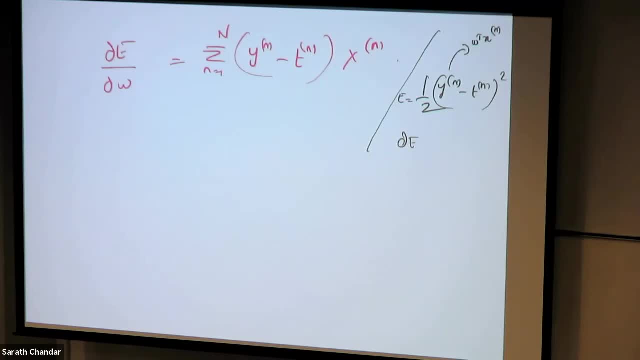 dou E. this is the error function okay, The least square. So dou E by dou W was basically Y of N minus T of N right. Two cancels multiplied by you, differentiate Y of N, you get just X of N right. 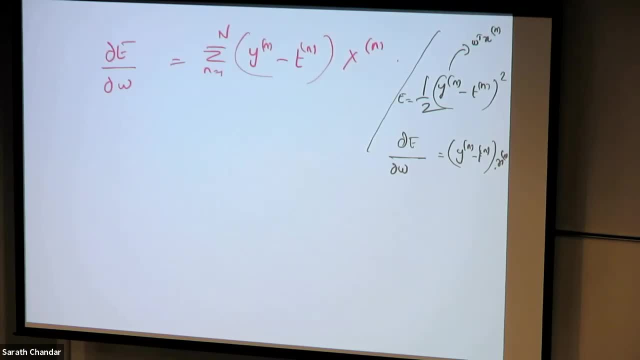 So this is exactly the same gradient equation that we had for, you know, the gradient descent: least squares. okay, Now so is this a coincidence that, like we have two different error functions like least squares and maximum likelihood, and it so happens that they have similar gradients? 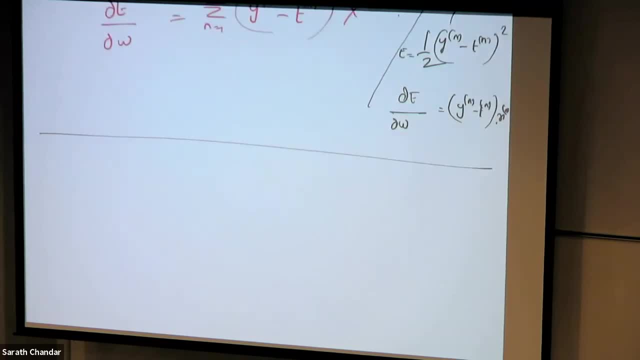 right. So now, this is not a coincidence, okay, So there is some connection between maximum likelihood and least squares, okay, So let's look at that now. So, connection between maximum likelihood and least squares: So if you think about it, least squares is not a probabilistic approach, right? 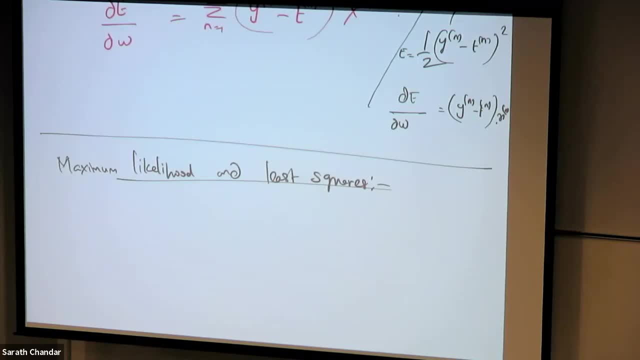 There is no probability involved in least squares. You just compute this mean squared error, you compute the gradient and then you get some W right. On the other hand, like with maximum likelihood, you have some probabilities and you're trying to estimate the likelihood right. 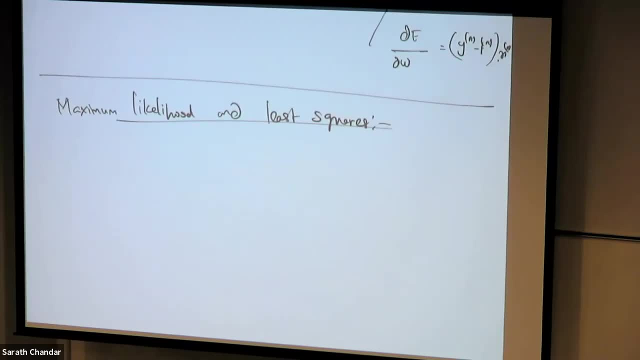 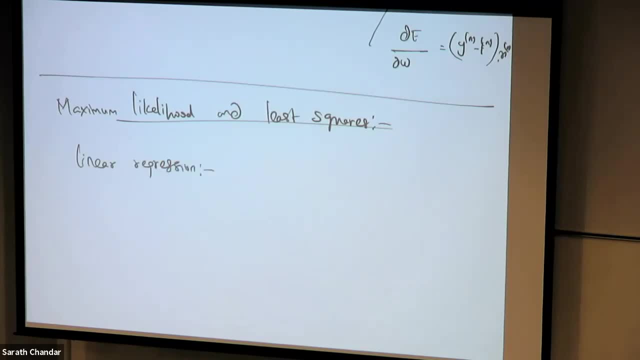 Once again, but from probabilistic perspective. okay, Now assume that in linear regression, your target T, instead of being a deterministic function of X, like instead of being just Y of X, given W. okay, has some Gaussian noise added to it? okay. 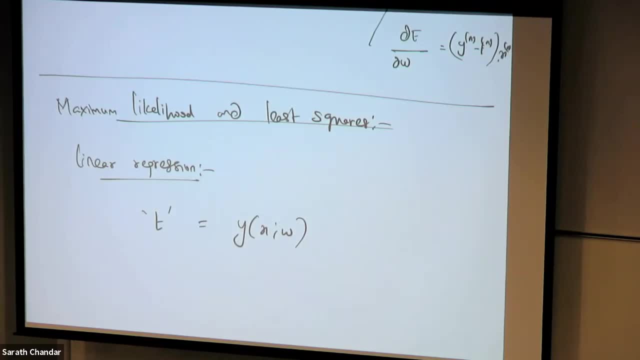 My target is going to be Y of X. come on, X given W plus some epsilon, where epsilon is a Gaussian with zero mean, and beta-inverse variance. Beta-inverse is basically precision, which is inverse of variance. okay, So you can put variance there if you want, okay. 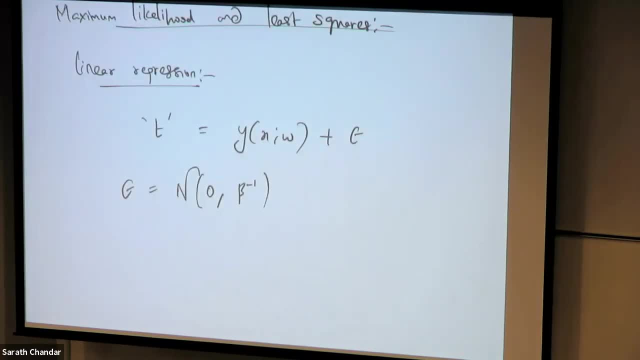 Now we have a probabilistic problem, right? So like we have a probability distribution over the target in regression, okay, Which means one can ask: what is the probability of T, given my input, X and W and beta, right? 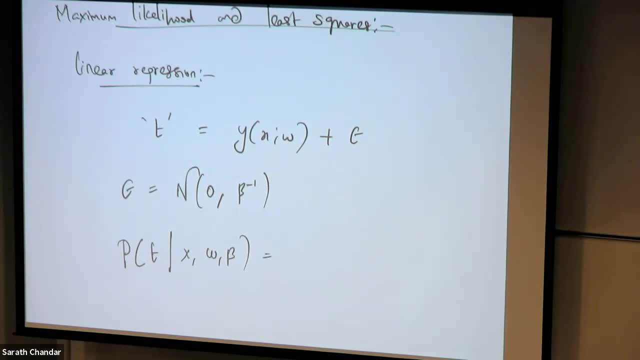 Now this is going to be a Gaussian which is centered around the target. okay, So it's going to be a Gaussian of T given Y of X given W. beta-inverse. It's a Gaussian with mean being Y of X given W. 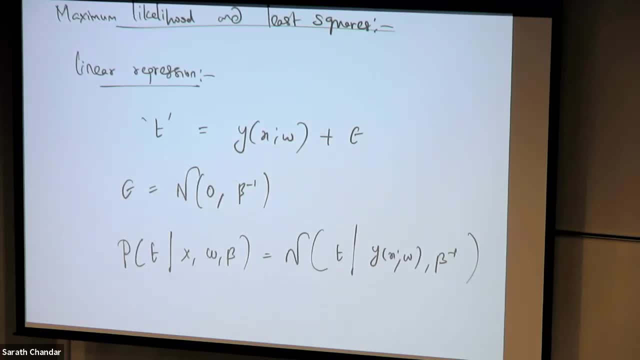 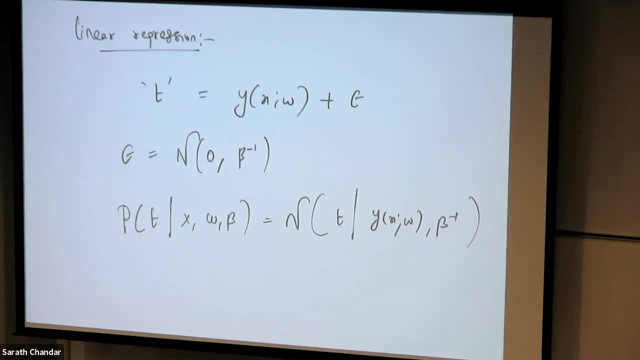 and variance being beta-inverse. We're clear Now. now I can actually do maximum likelihood for linear regression, right, So I have. I have a probability for a target given input, right. So now this is a probabilistic model. 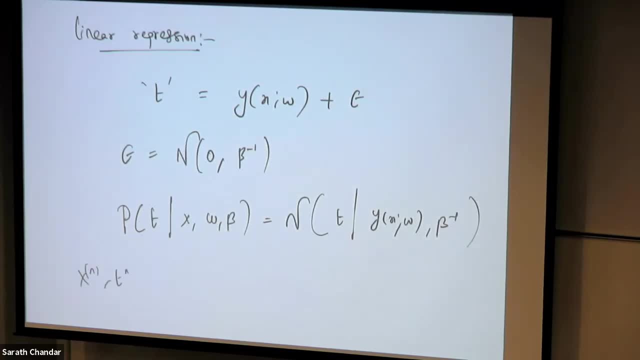 Now I can take a data set which is a bunch of X and Tn, where n is equal to 1 to capital Tn, and maximize the probability like: find the parameter subset that maximizes the probability right. So now the probability of T given X, W, beta. 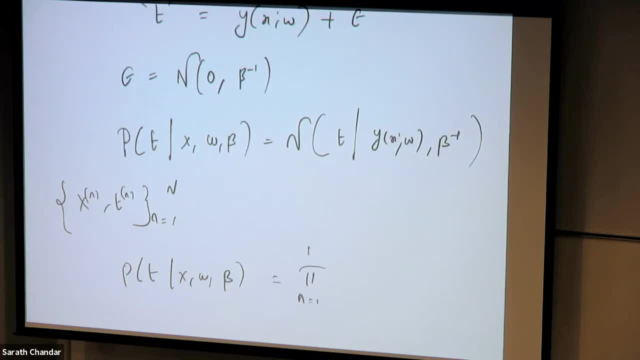 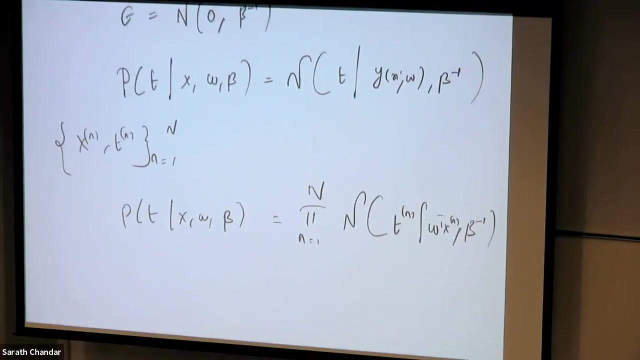 is given by product over n is equal to 1 to capital N. a Gaussian of T of N, given W, transpose X of N comma beta-inverse. Is that right? Okay, Now, as usual, like we can do long probability. 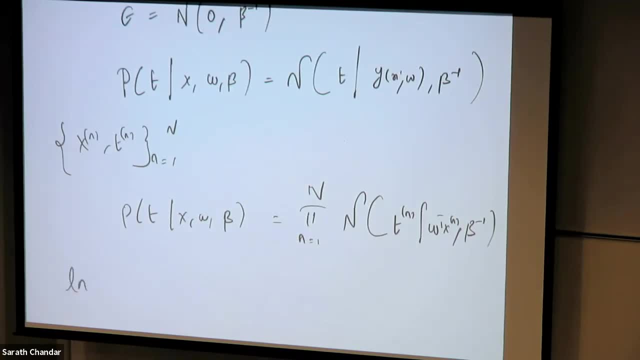 Instead of just probability. So I'm going to do long P of T. given X: W beta is equal to summation over n is equal to 1 to capital N. long normal distribution: given W: transpose X beta-inverse Right. 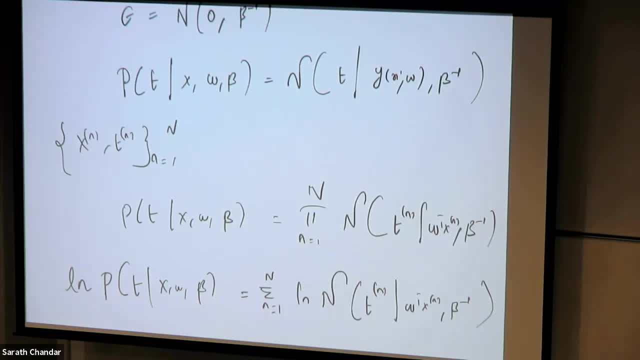 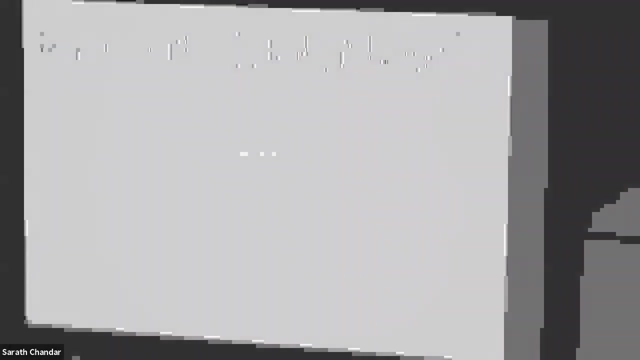 Okay, So let me just take this to the next page. Okay, Now this is actually equivalent to okay, so I think I moved too fast. Now the video is not working. Let's just wait for a few seconds. 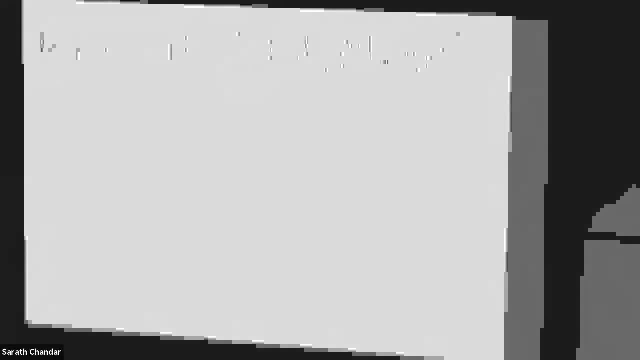 Well, this is the problem with the camera. Okay, So now we know what is the distribution function for Gaussian right, Like it has a bunch of terms in it, Like. so now I'm going to directly write the equation. 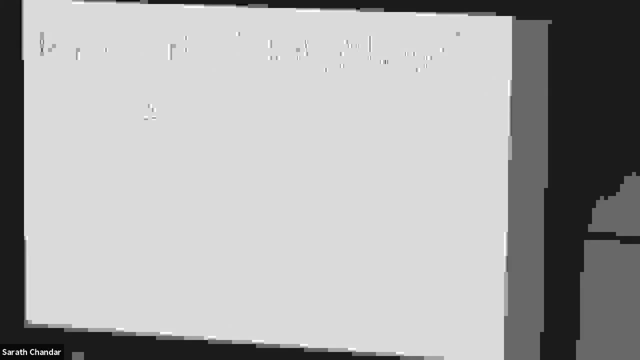 after applying ln. So it's basically n over 2 ln beta minus n over 2 ln T pi minus beta times over 2. summation over n is equal to 1 to capital N, capital N, T of n and the returns for X of n. 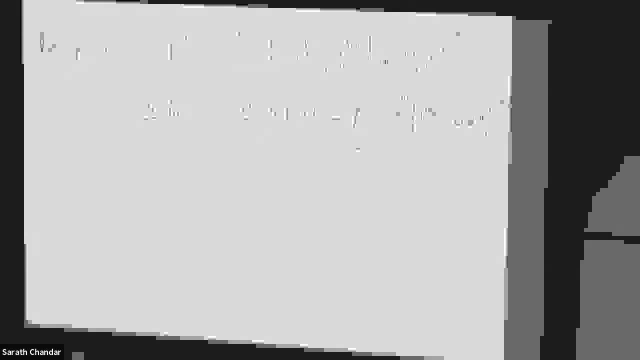 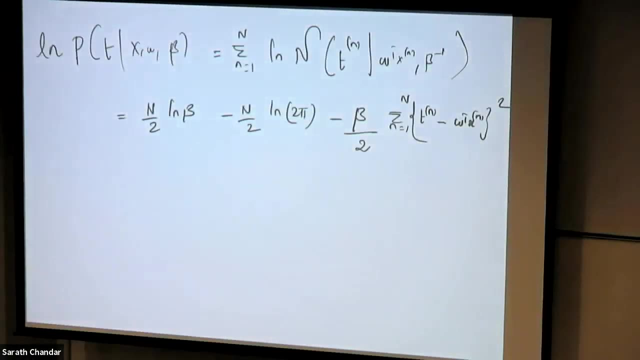 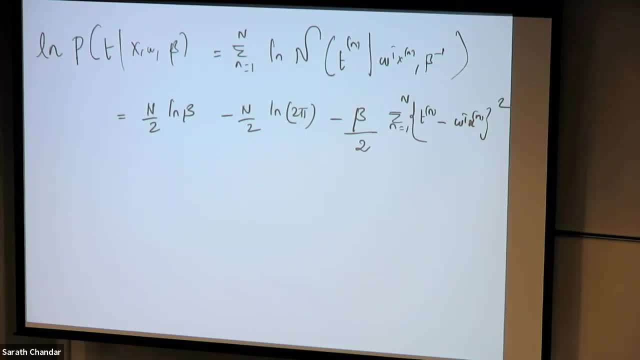 multivariate Gaussian, Like I applied ln. So then you divide things into three parts. This is what you have. Okay, So given that the mean is W, transpose X of n. Now we want to maximize this log probability, right? 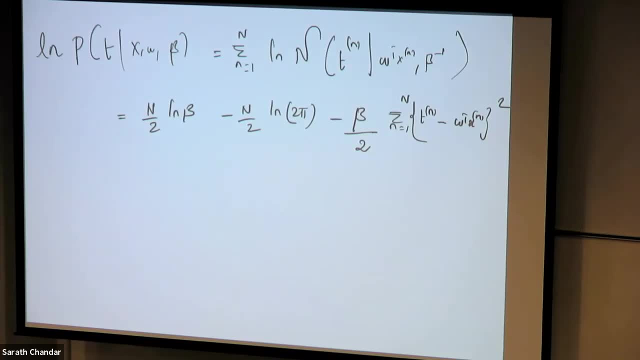 Or minimize the negation of this, When I want to maximize, like when I want to find W which maximizes this probability. well, you can notice that the first term does not have any W in it. The second term, the third term, does not have any W in it. 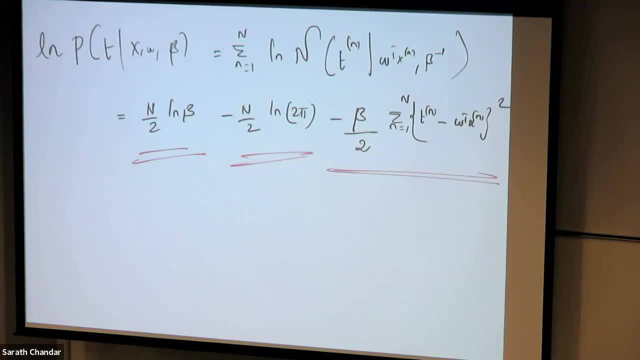 So only this term has W in it Right Now, if you just consider this term right, You want to maximize this term, which is equivalent to actually minimizing plus beta by two. summation over n is equal to one to the capital N. 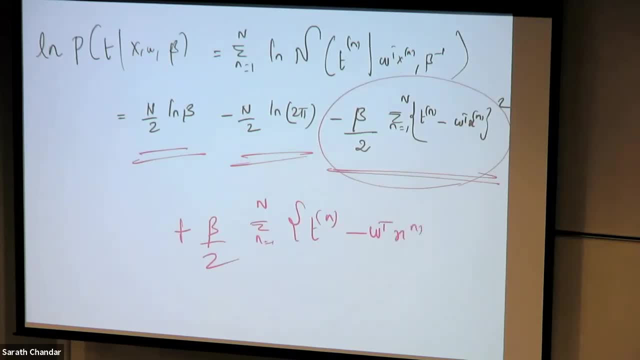 T of n minus W. transpose X of n plus W, Right. So you either maximize this or you minimize this, Right? So now you can see that maximizing the log likelihood is actually equivalent to minimizing. this looks like what Mean squared error, right. 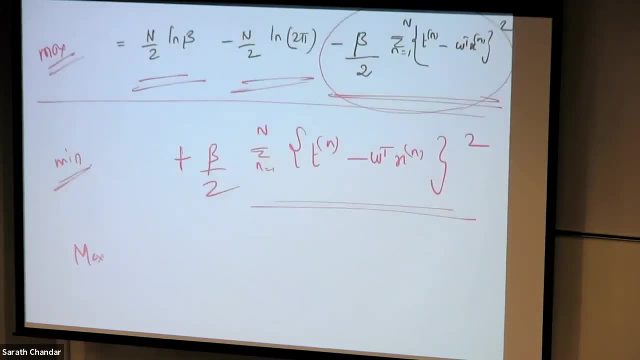 So maximizing log likelihood is equivalent to minimizing least square. So if you do least squares error, if you make Gaussian assumption for noise, if you assume that your target variable follows a Gaussian distribution, then when you do least squares you're essentially doing maximum likelihood. 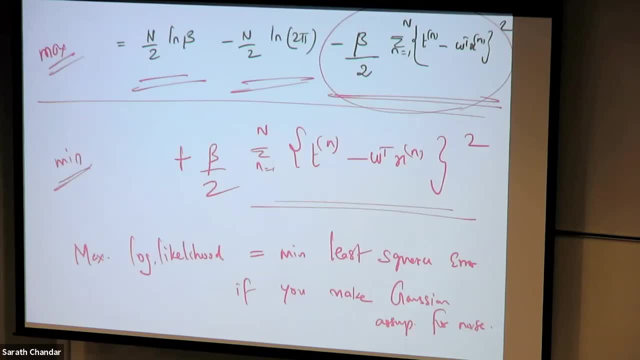 Is that clear? Any questions? Any questions in the Zoom? Okay, Now we can actually make a lot of connections with the past. Okay, So now, if you think about least squares, what is the optimal solution for least square? 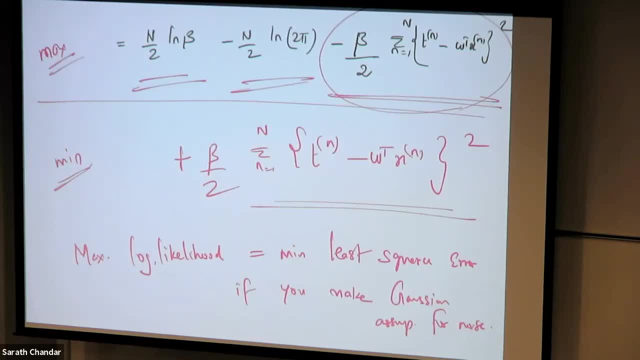 Anybody. What is optimal solution for least squares? Expected value: Expected value of T given X. right, So I hear answers from only few students. Maybe we should have had a midterm exam. Okay, So the optimal value that one could achieve for least squares is P of T given X. 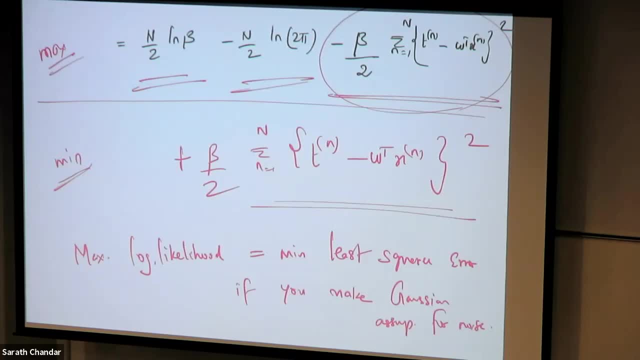 Right Now. this connection tells us that P of T, given X, is actually a Gaussian, which means that it is unique Right, Which means that it is unimodal. There's only one mode for Gaussian right, Which is a very restrictive assumption. 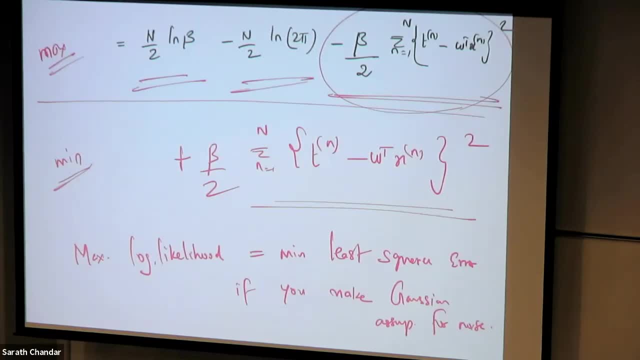 Because in reality, for most of the classification problems, you will have multiple modes in the distribution. Okay, So you will not have a simple Gaussian for the class. Okay. Now this actually kind of helps us to understand why least squares is actually a bad classifier. 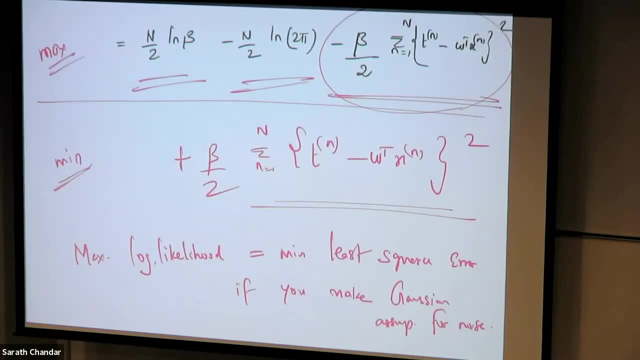 Even though it was our first classifier. now you understand that it is a bad classifier because it makes sense. It makes this very strong assumption that P of T given X is unimodal. Okay. On the other hand, like for most of the binary classification problems, or 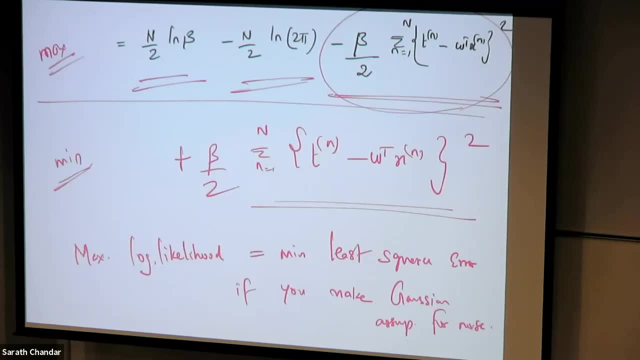 K class classifications problem that we are going to see. we will not like. the data will not respect the Gaussian distribution, Which is why we need something else. Is that clear, Okay? So any questions so far? So I think what we have done so far is like: 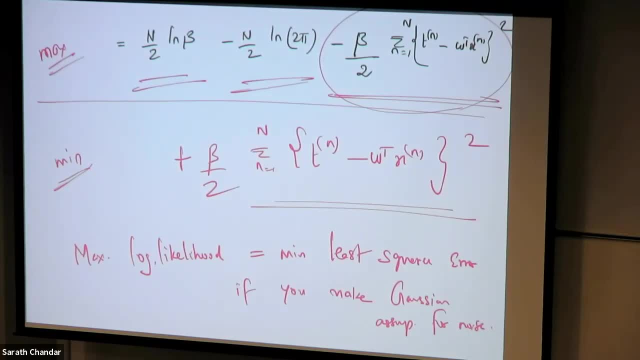 I introduced logistic regression And we did gradient descent for logistic regression And we also saw connections between maximum likelihood and least squares. Yeah For classification, Okay, Not for regression. So in the case of classification, if you do least squares, 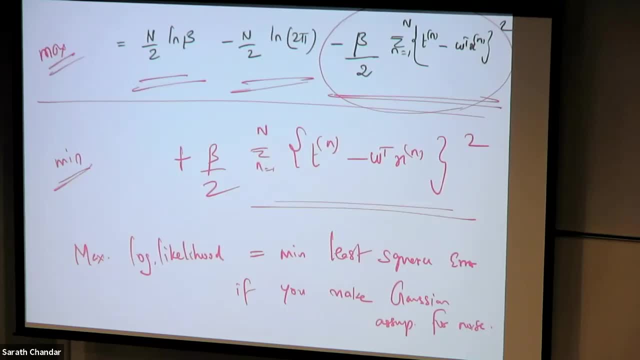 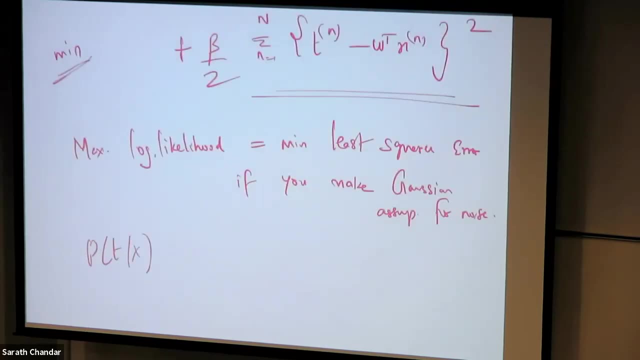 then you are making this assumption that P of T given X is unimodal. Like so, P of T given X. you assume that it is going to be something like, something like a Gaussian. Okay, Like so, Exactly Gaussian, because that's what you are assuming. 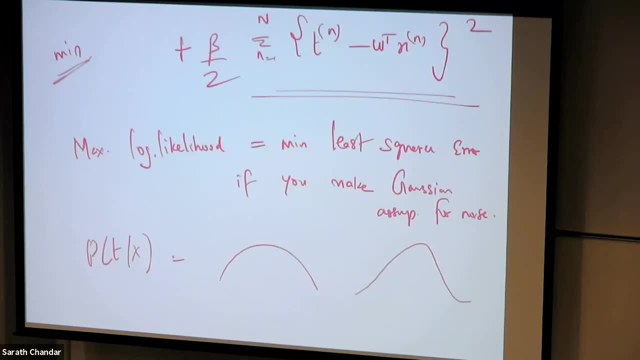 Right, Maybe I drew bad Gaussian here, Like something like this: Okay, On the other, in reality, the data might have complex distributions, Right? So we don't know that. So most often, the data is going to have complex distributions. 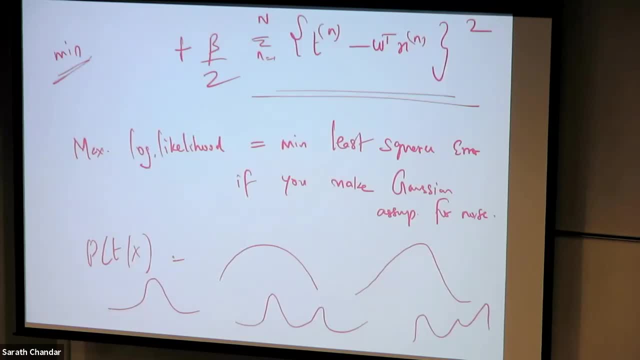 Yeah, Do they have the same closed form solution or no? No, So, as you can see, we have closed form solutions for regression, but we don't have closed form solutions for logistic regression. Okay, So, after the break.